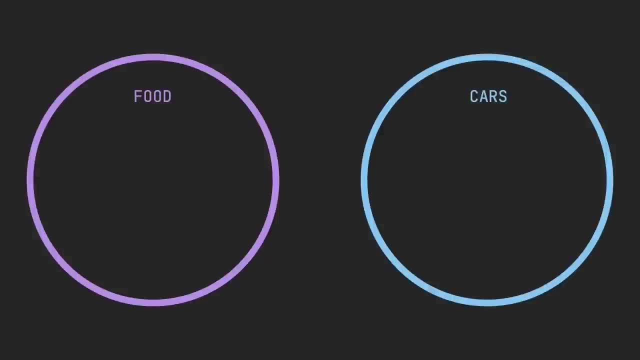 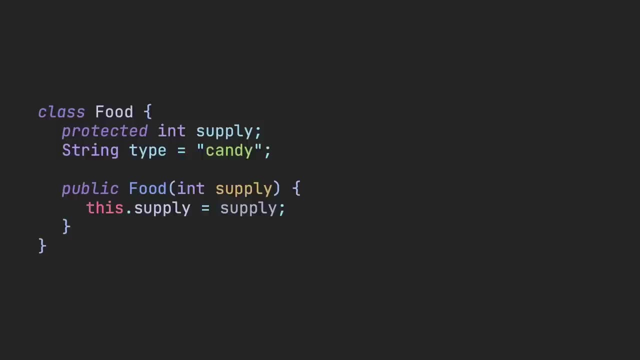 be considered a blueprint to instantiate objects. Classes usually represent a broad category, such as cars, animals or any other encompassing field. For example, if we have a class food with attributes supply and type, we can now create as many objects of food as we like. 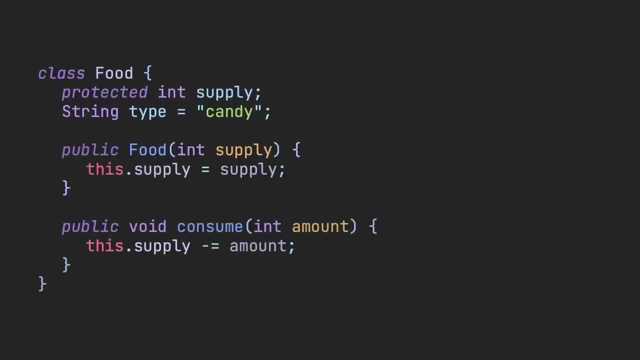 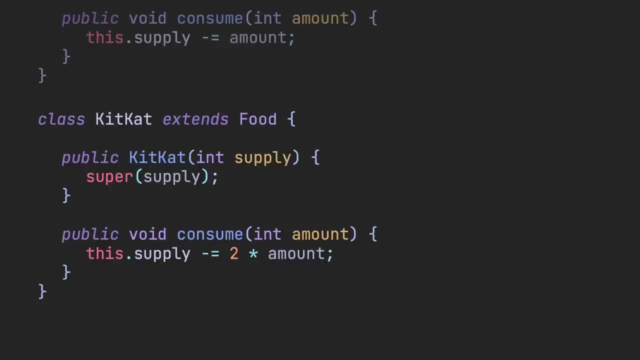 To add some more functionality. the class food can have methods. Most classes are even more powerful than they look like as they can be extended from to make more subclasses. Here KitKat can extend from food. With KitKat everything is the same, except the consume function is overridden. 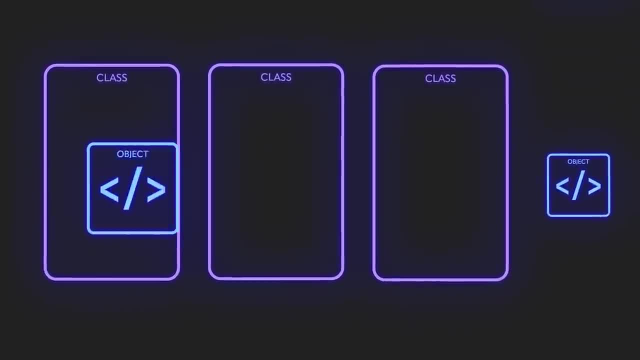 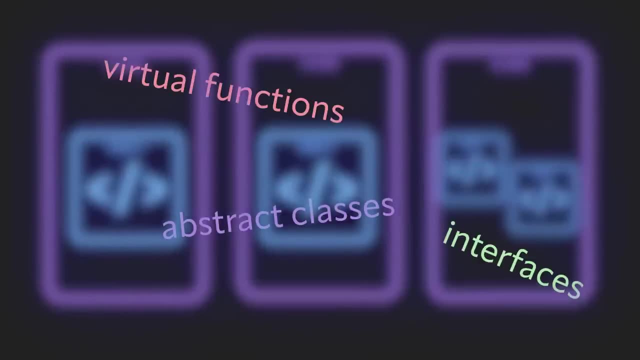 While this specific example is extremely simple, an object-oriented design allows for flexible code reuse. Object-oriented programming can be made more robust with features like abstract classes, interfaces, virtual functions, multiple inheritance and more, but that's beyond the scope of OOP. 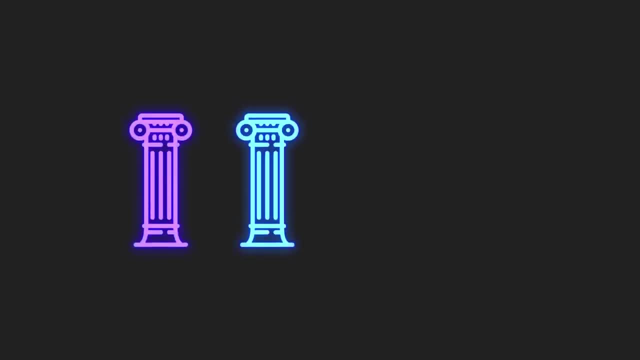 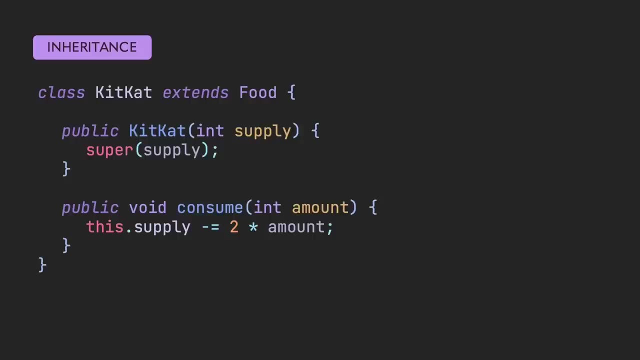 Something you'll probably hear a lot related to object-oriented programming are its four pillars. These are inheritance, polymorphism, encapsulation and abstraction. Inheritance is what I mentioned earlier about KitKat extending food. KitKats are still a type of food, so 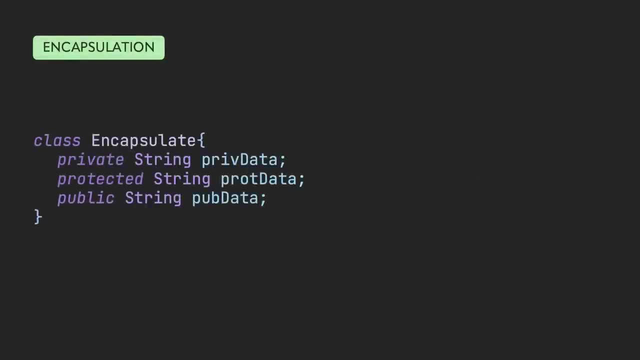 they should be able to take all the properties of food. Encapsulation allows classes to manage how they hide data, allowing access through either the class itself or a function. For example, if we have a class for a person we wouldn't want their address or ssend to. be public. Otherwise we'd be able to take all the properties of the food. For example, if we have a class for a person, we wouldn't want their address or ssend to be public. Otherwise, we'd be able to take all the properties of the food. Otherwise, any other class would. 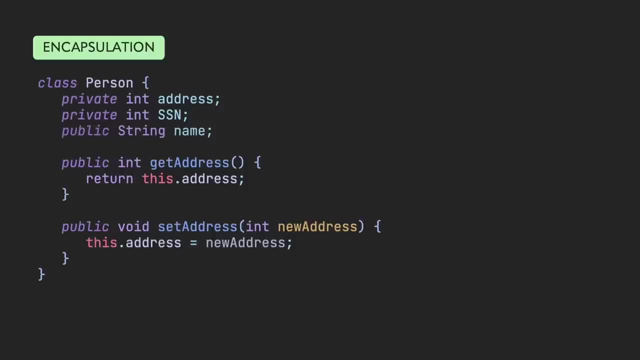 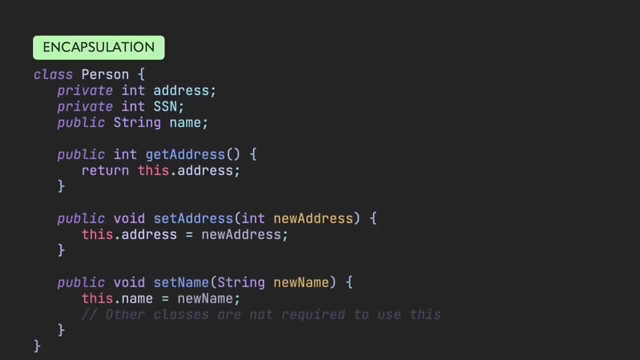 be able to access and potentially change those properties. On the flip side, something like your name could be public. as that data isn't as sensitive, The best practice is to declare any variables as private, so nothing outside the class can affect it, unless it needs to be public. 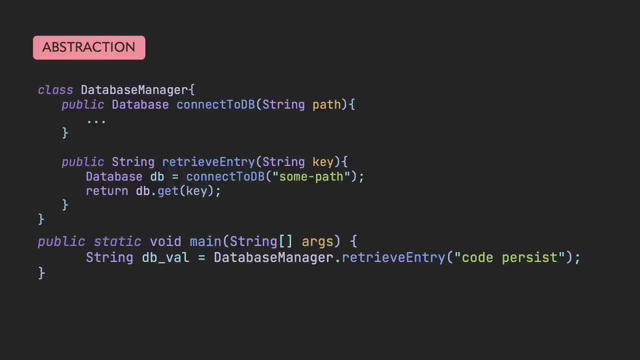 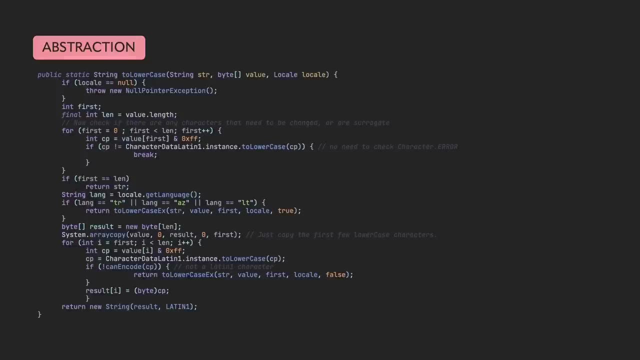 Abstraction is similar to encapsulation. however, it's less about data safety but rather for ease of use. If we have a string and we want it to be lowercase, we can just call it the toLowercase function, as we don't need to know exactly how the string will be made into. 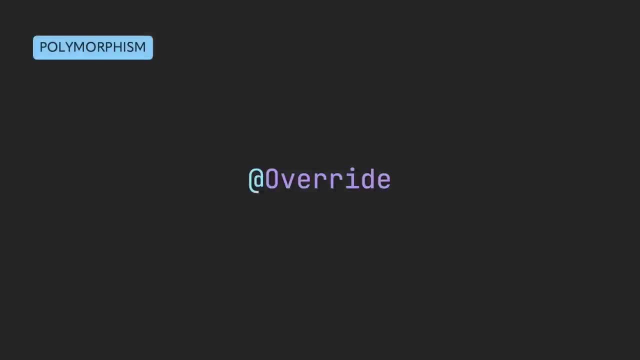 lowercase. Polymorphism is also similar to inheritance, except it's about modifying behavior rather than taking properties. In my earlier example, polymorphism is used when we override the consume function. Object-oriented programming is not perfect and it has its issues. 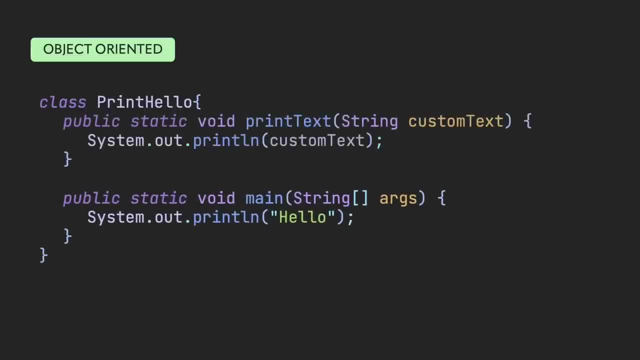 First of all, the code made with object-oriented patterns will generally be longer than other styles. There's just more boilerplate code to write, and if the project doesn't need all the boilerplate, there'll be a lot of extra unnecessary code. 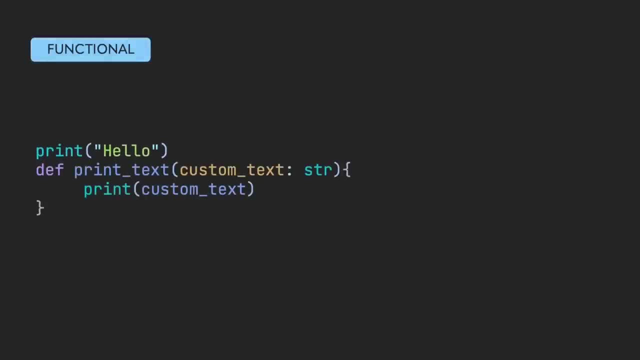 That's where functional programming can come in. I apologize in advance if I get something wrong with functional programming, as I don't have a great deal of experience in it. That being said, reading and writing well-written functional programs feel great, as they can. 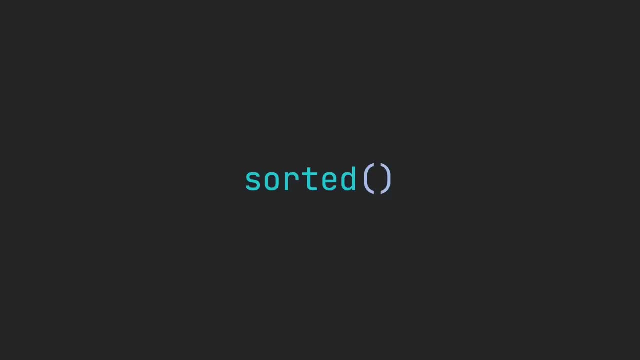 be extremely elegant. The main idea with functional programming is that we use functions as our primary building block, as opposed to classes and objects. The functions are usually pure functions, avoiding shared state, mutable data and side effects. For example, if we have a function that adds two variables and changes a global variable. 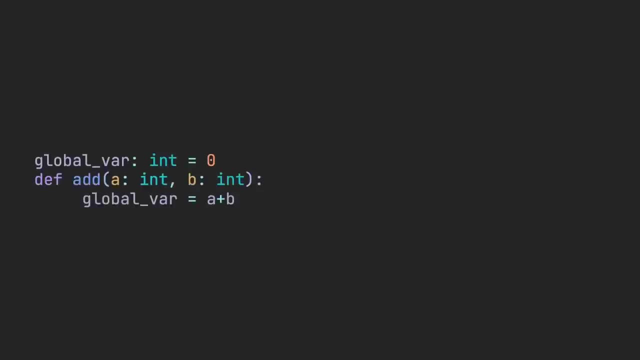 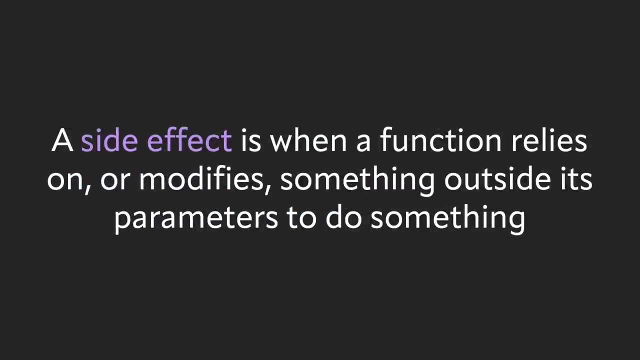 to the sum. This would not be a functional program. It would be a functional programming concept, as we introduced a side effect. The side effect was caused by altering a piece of data beyond our scope, which is the function. Side effects are something developers avoid, as they can cause bugs that are completely 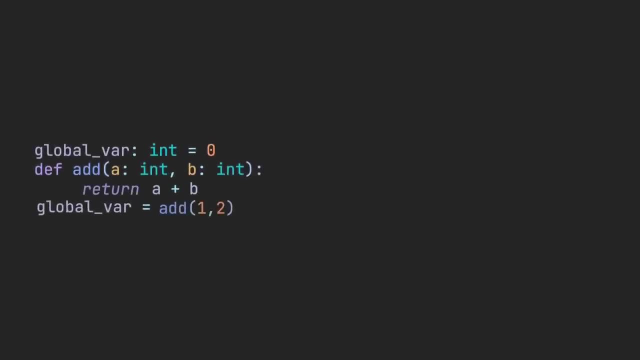 unexpected. We can make the function pure by not altering the global variable. Another concept of functional programming is that data is immutable, because mutable data can also cause side effects. Instead of having shared state and mutable data, we can alter data by using other functions. 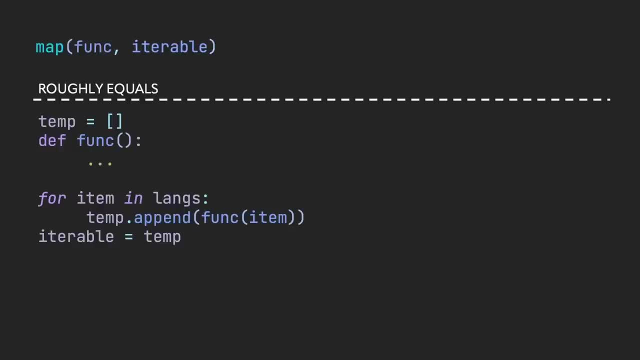 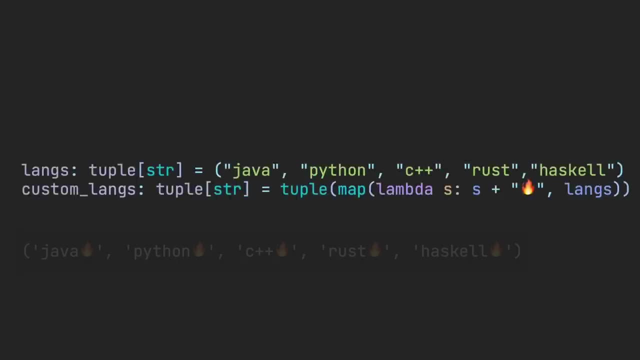 such as map. All map does is run a function non-everywhere. In this case, we just append a fire emoji to the end of each string. Map is also an example of a higher-order function, as it's a function that takes another function. 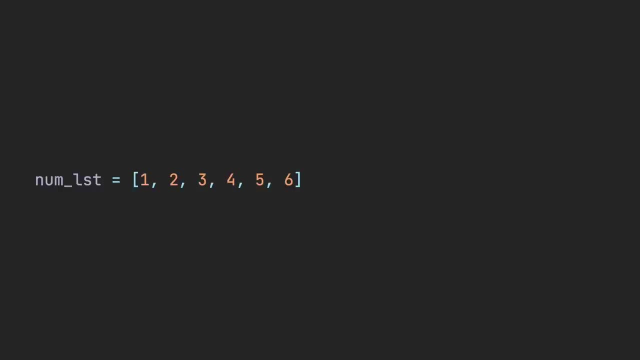 as a parameter. Functional programming has many benefits that object-oriented programming doesn't have. You can get these beautiful or ugly one-liners, depending on how you like your code to look. It's also far easier to track down bugs, as a bug should only be contained within one. 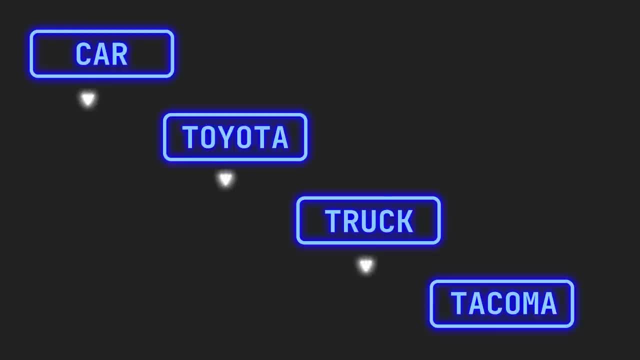 function and won't have you jumping through 10 different files and nested objects. If you have any questions, feel free to ask them in the comments below. Thanks for watching. Although functional programming seems like a developer's dream, with smaller projects it can be considerably harder to scale up in certain cases. 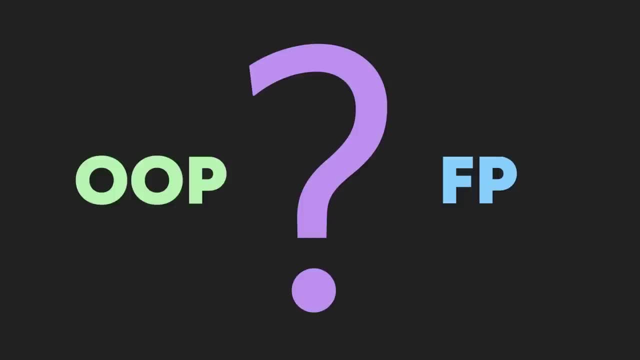 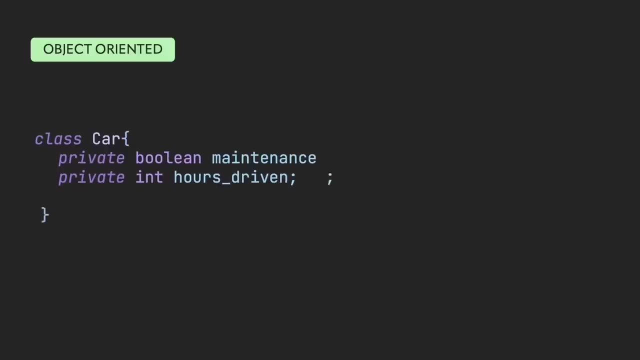 This is because modeling a problem with functional programming is not as easy as it is in object-oriented programming. For example, take a car that needs maintenance on a certain date. In this case we can just have a car object with an attribute for when it needs maintenance.